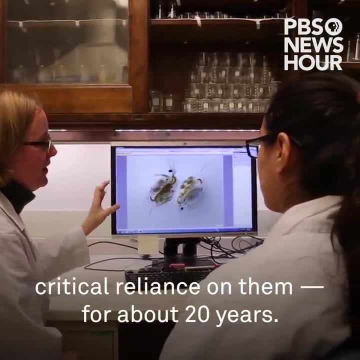 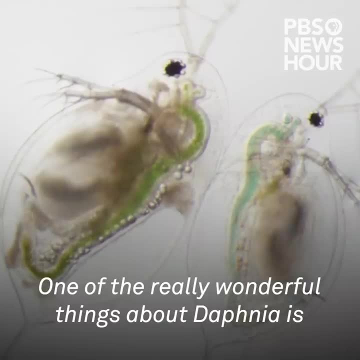 with the tiny creatures and our critical reliance on them for about 20 years. I had no idea daphnia existed until I was a college student. One of the really wonderful things about daphnia is they're transparent and that makes them really beautiful to look at. You can actually see their gut with. 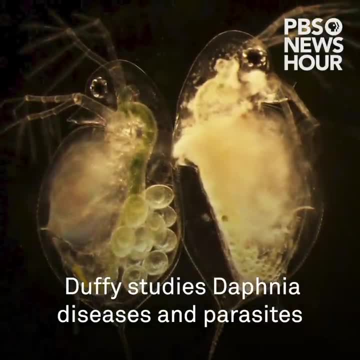 all the different colors that they have and they're really beautiful to look at. They're really beautiful to look at. You can actually see their gut with all the different colors of algae in it. Duffy studies, daphnia, diseases and parasites in the lab, Like humans, the microscopic. 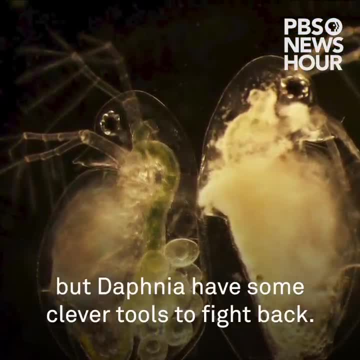 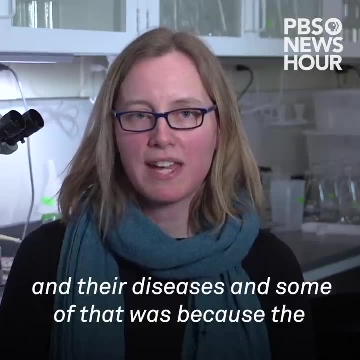 creatures experience outbreaks of fungus or bacterial infections, but daphnia have some clever tools to fight back. We started this research interested mainly in daphnia and their diseases, and some of that was because the daphnia are so ecologically important. 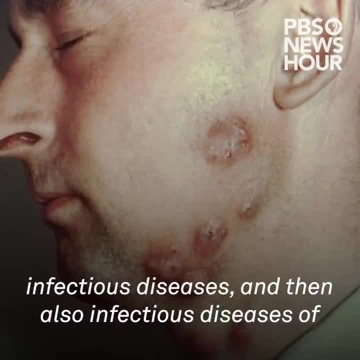 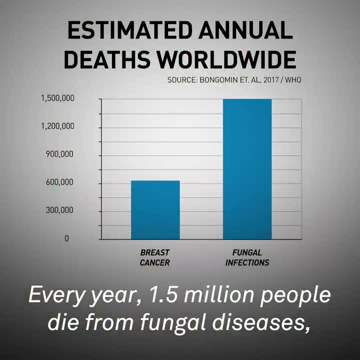 But as we've done the work, we've realized that it also is relevant to human infectious diseases, and then also infectious diseases of wildlife and crops. Every year, 1.5 million people die from fungal diseases, which is three times the number that die from breast cancer. 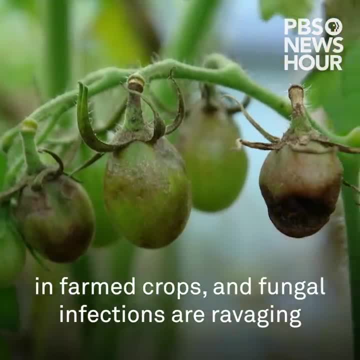 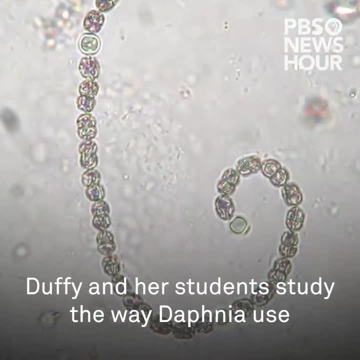 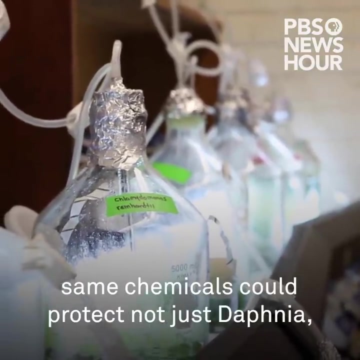 Fungi also cause two-thirds of the diseases in farmed crops, and fungal infections are ravaging vulnerable populations of bats, frogs and snakes. Duffy and her students study the way daphnia use chemicals from the algae they eat to protect themselves from fungal diseases. They want to know if those same chemicals could protect not. 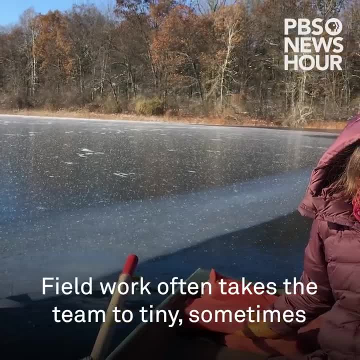 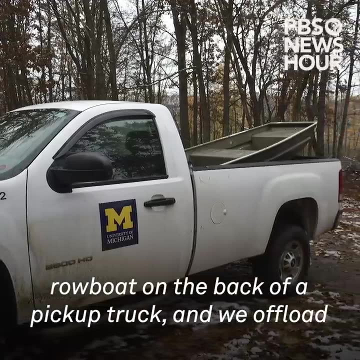 just daphnia, but other kinds of life too. Fieldwork often takes the team to tiny, sometimes frozen, Michigan lakes. When we drive out to the lake, we're going to the lake, We're going to the lake. drive out to the lake with our little flat bottom rowboat on the back of a pickup truck. 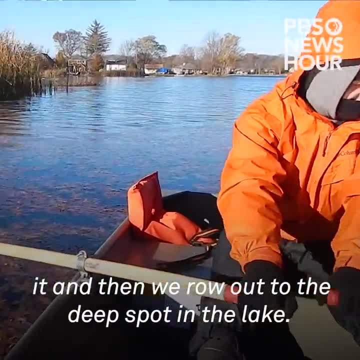 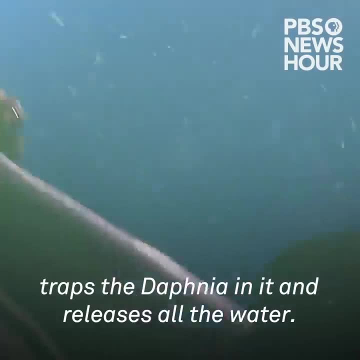 and we offload it. and then we row out to the deep spot in the lake and we use a plankton net, which you can think of as like pantyhose, and we pull that through the water and it traps the daphnia in it and releases all the water, And then we put that in a bottle and we can bring it back. 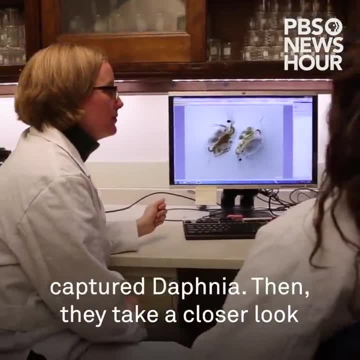 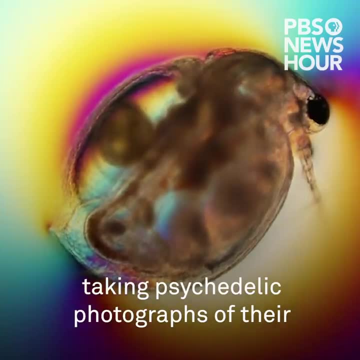 to the lab. That's where Duffy and her students can count their captured daphnia. Then they take a closer look under a microscope, inspecting them for infections, checking what they might be eating and taking psychedelic photographs of their tiny prizes. Recently, the lab has found three. 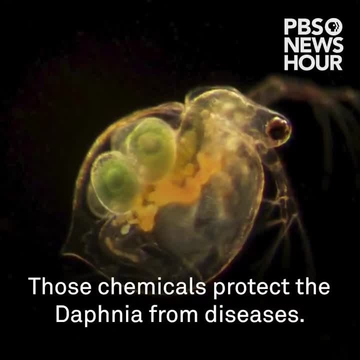 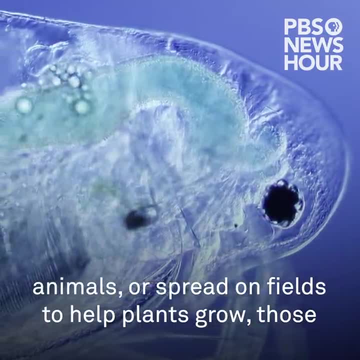 fungus-fighting chemicals in the foods that daphnia eat. Those chemicals protect the daphnia from diseases. If they can be developed into medicines for people and animals or spread on fields to help plants grow, those chemicals may someday protect us from these dangerous diseases.